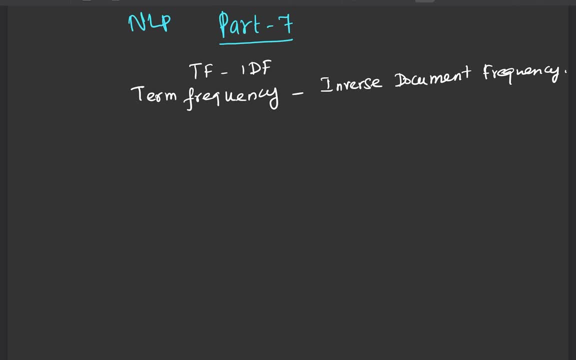 first term, term, frequency, which measure how relevant the document is related to the topic. So here in our example, the same example we are doing, We will take the sentiment analysis. There are two sentences. The sentence one is: I like the movie. The movie was awesome. 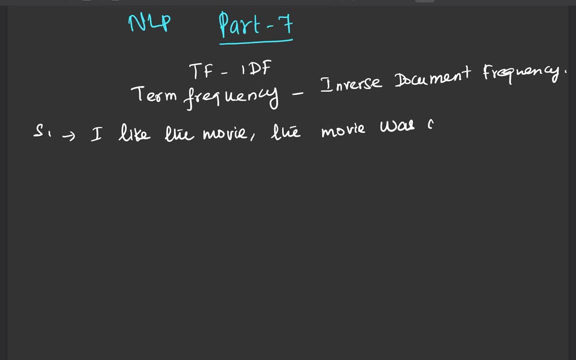 And the second sentence is: I do not like the movie. The movie was boring. So, after applying our feature engineering data pre-processing, It is not feature engineering, It is data pre-processing. So what we do, we will remove all these top words and irrelevant words and do some kind of stemming and lemmatization. 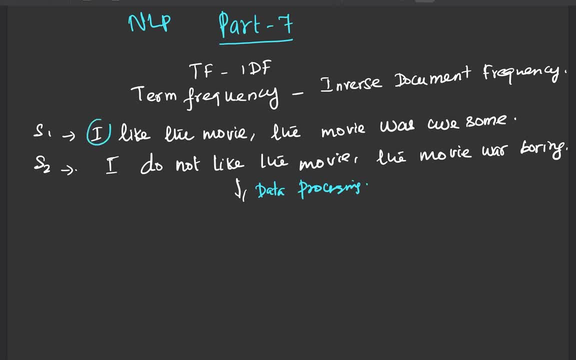 After doing those, the words I like, the movie, The, the was. These words will get removed. I do the, the was. These are all not required for our sentiment or classification, So we are trying to see whether it is a positive sentiment, whether it is a negative sentiment or not. 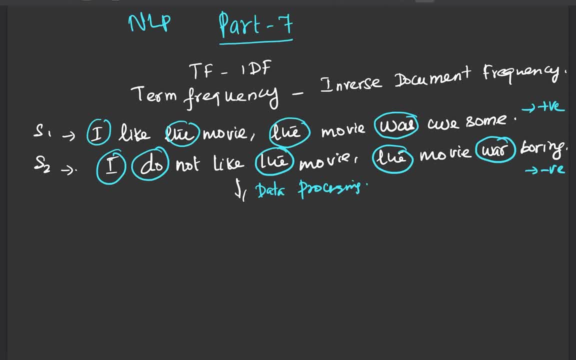 So after we do the feature engineering, the data pre-processing, Our feature That document would like would look like this: The first one for the sentence S1.. The corpus would have this like: Movie Again movie. 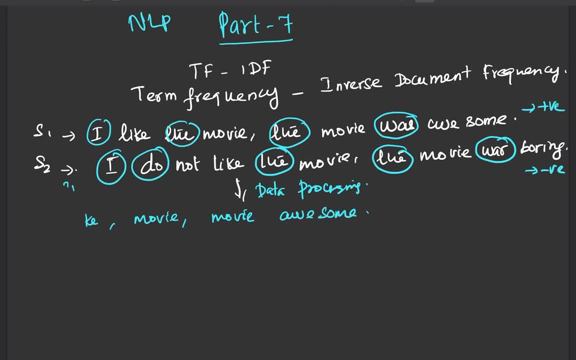 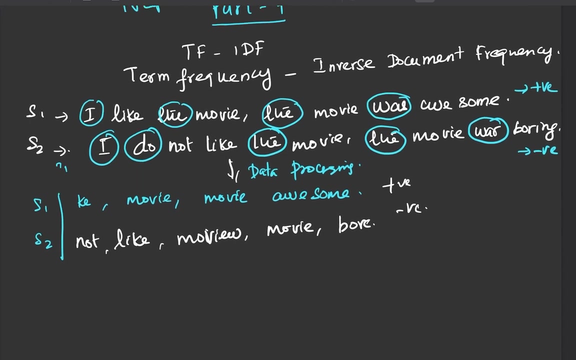 Awesome. This is sentence one. Sentence two: This is Not Like Movie, Again, movie Bore. So here, this is positive sentence, This is negative sentence. Then how we interpret this term frequency in this context? 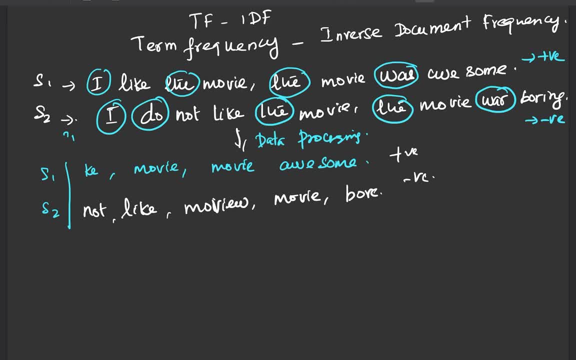 Term frequency is just trying to understand what is the frequency of each word in the given document, How relevant the word is in the given document for the given context. So this would look at how frequently the word is appeared. The movie appeared two times. 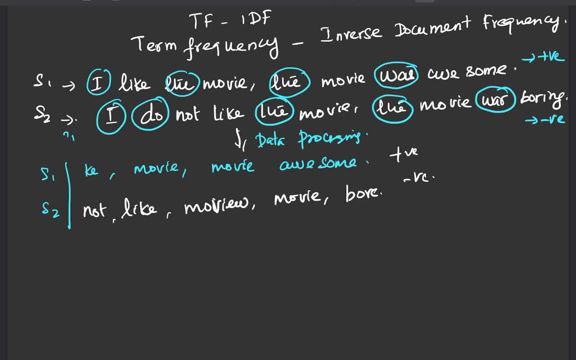 And the awesome appeared one time. So this term frequency would suggest that the word movie is more important than awesome and like. But it is not true. Then there is another method to calculate, which is IDF- Inverse Document Frequency. 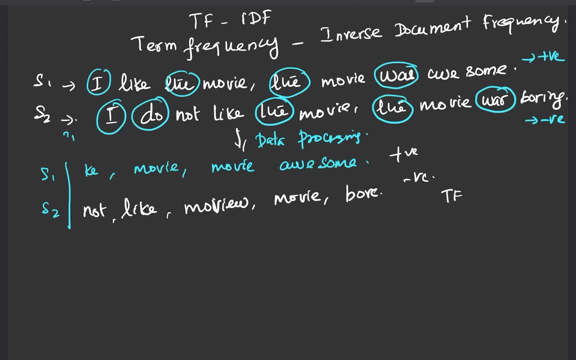 So this is a kind of locally searching. This term frequency is locally searching inside a document And see how relevant the word is inside the document. Again, another one is IDF, which is searching across all the document And see how many times the word appeared across the document. 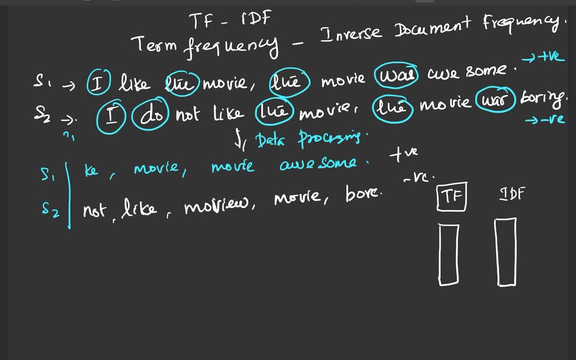 And inverse of that frequency. So when you take the word movie, The term frequency would show like this: So here the total number of words are 4.. So the term frequency- how we calculate term frequency- is Denominator- is total number of words in the document. 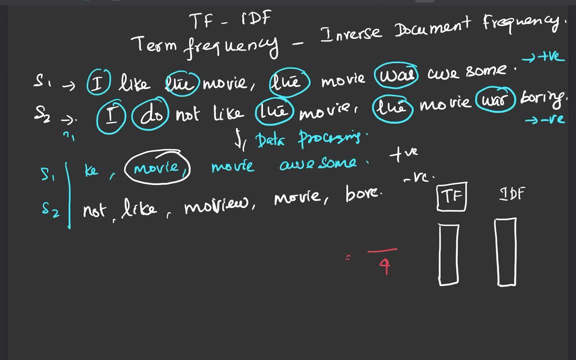 1,, 2,, 3, 4.. Out of which I am calculating this value for word movie. For the word movie, the term frequency TF is 2 times out of 4 times. So this would be this much. 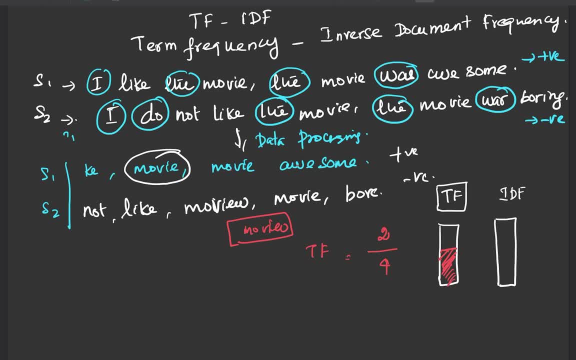 At the same time how we calculate inverse document frequency. So before seeing inverse document frequency, we will see what is document frequency. So, like term frequency, Document frequency is looking at the total number of documents, How many documents we have. 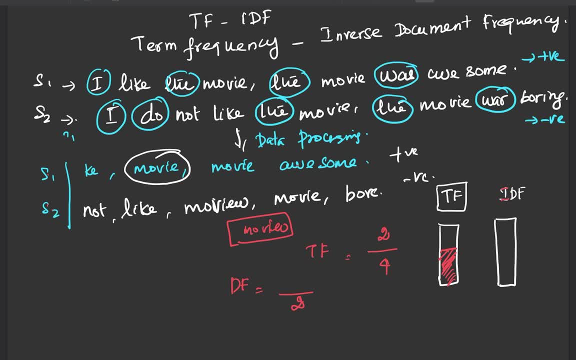 Here 2.. Out of 2, how many documents have this word movie 2.. So inverse document frequency is just inversing. So here, since 2 and 2 are same, We will not see any difference. Maybe look at another word: awesome. 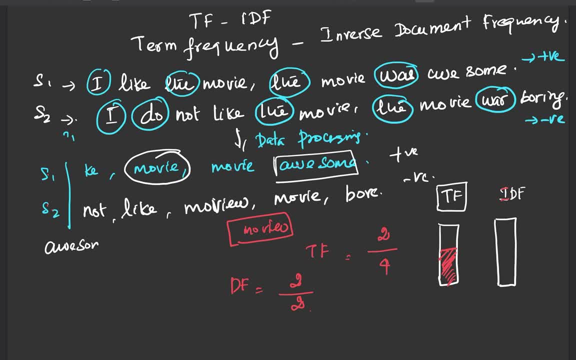 So for awesome the term frequency, TF is just locally searching within the document. Denominator is 4, total number of words And numerator is 1.. Only one time this awesome appeared. Another one is inverse document frequency. Here just first measure this document frequency. 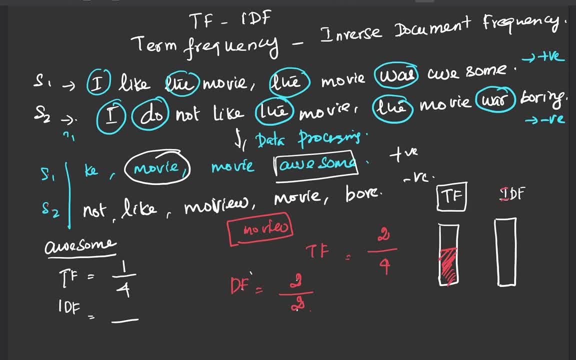 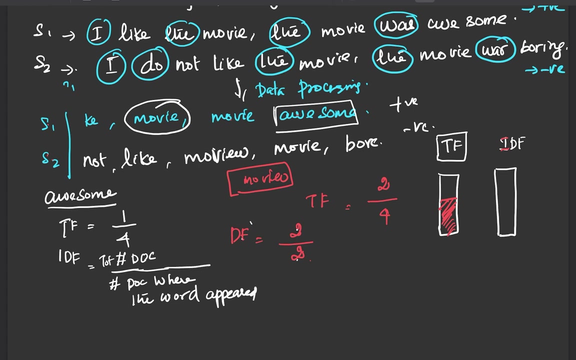 Denominator is total number of document And how many times this appeared on the document. Here in IDF the numerator is total number of documents And this is total number of document- Number of documents where the word appeared, So, which is 2 document. 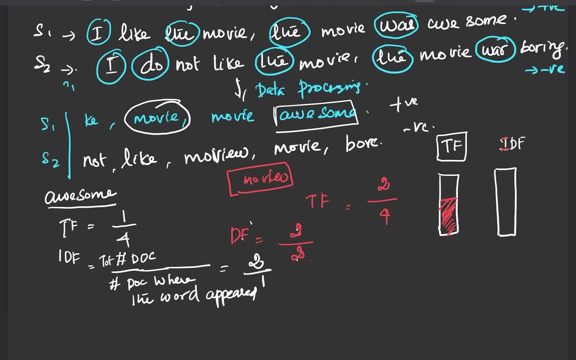 Out of 2, the awesome appeared on one time, So here we need to take log of this value. This is called as inverse document frequency. So what is inverse document frequency? for this word, movie Document frequency is 2 by 2.. 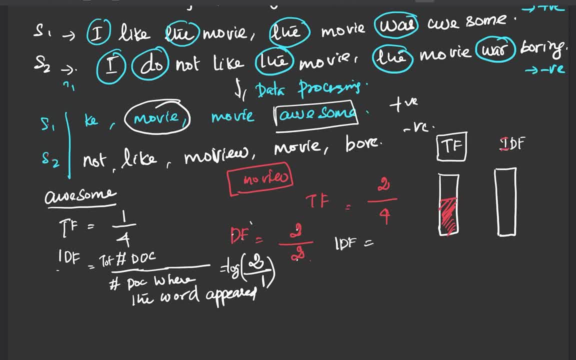 And inverse document frequency. for this word movie is just taking the log ratio of 2 by 2.. Which is actually how much? What is the log of 2 by 2?? It is log 1 which becomes 0. So the inverse document frequency is empty. 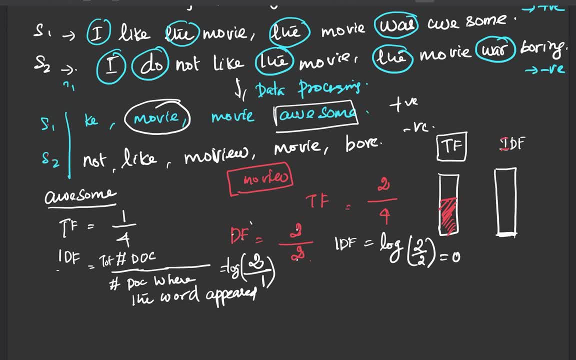 Here, no value here, And then what we are trying to do is we are coming up with a single number that represents the relevance of the importance of the word in the document. This is TFIDF. What we are doing here is we are just multiplying these two factors. 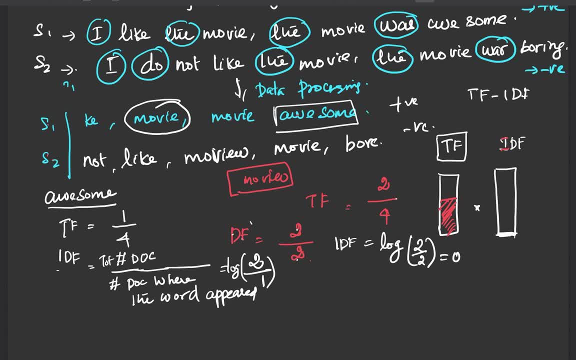 Here we got 2 by 4. This is 1 by 2. So the TFIDF value for the movie is 1 by 2 into 0. So when we multiply it becomes 0. This is pretty much what we want. 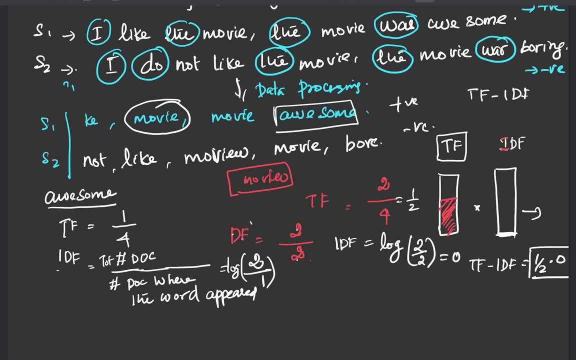 This is more relevant than bag of word methods. In bag of word methods it would be just looking at frequency of words, Frequency of words for a given word. So here, for movie, we would get 2.. For awesome, we would get 1.. 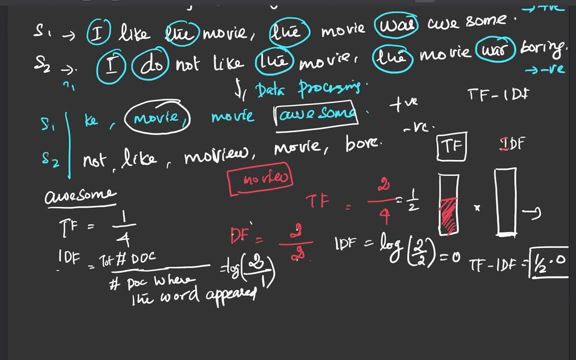 And for like, we would get 1.. But using TFIDF for movie, the overall value becomes 0.. Because this is not relevant? Because this movie is not only specific to the first sentence. It appeared on the second sentence as well. 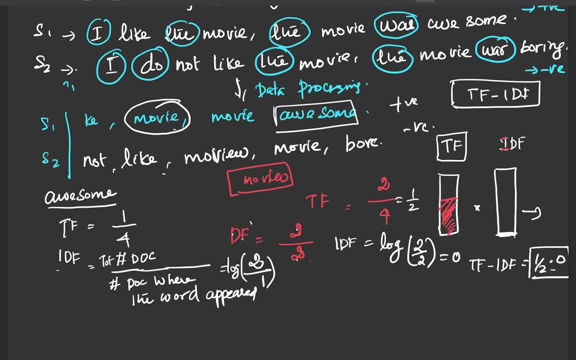 So, irrespective of the context, it is very common across all the sentences, So it is not giving importance to this word movie. So another kind of example is the words I, the, and those words will be appearing in across all the documents. 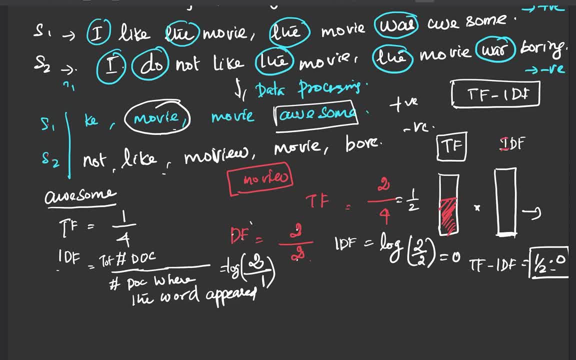 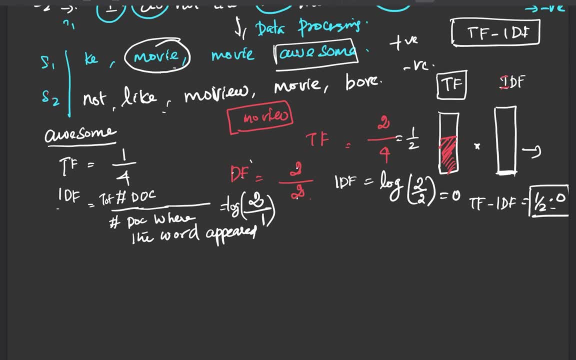 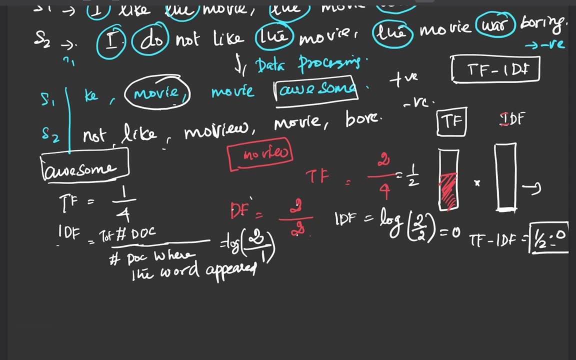 Even though that appears in across all the documents. those words are not important. Then we will calculate the same TFIDF for this another word. What is that word? Awesome, For this awesome word, we calculated this TF and log of 2 by 1.. 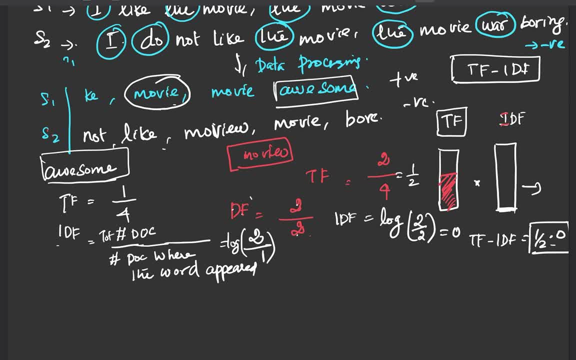 And we calculated this TF value And we calculate IDF value And then multiply TF values compared to this TF value. here it is 0.5.. But here it is only 0.25.. But even though it is 0.5,. 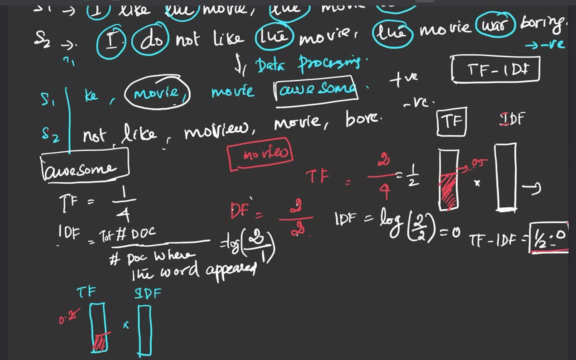 and the overall value when we multiplied with IDF, which becomes 0. Here we get some value for log 2.. When we multiply, we get some number. So this value is 0.5.. So this is how we can calculate the relevance of the word. 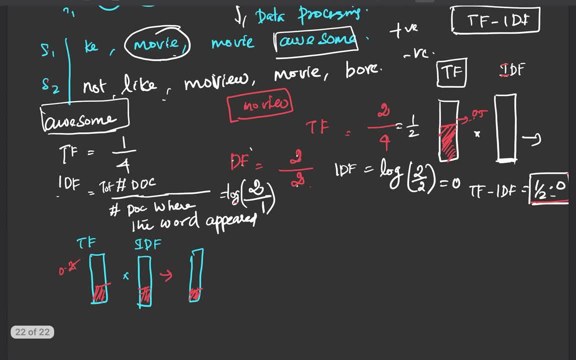 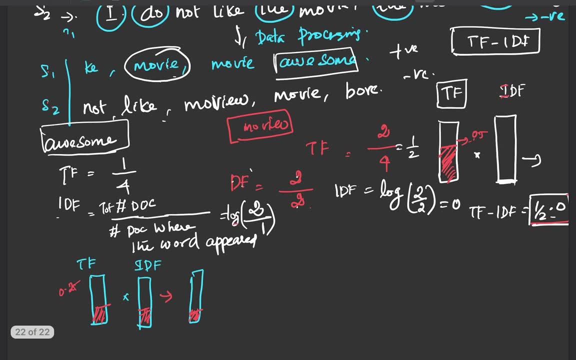 or importance of the word within the given document. So maybe for the entire feature extraction we will see how we can do. So. we have done this S1, S2.. Now we will see how we can extract the features using this TFIDF. 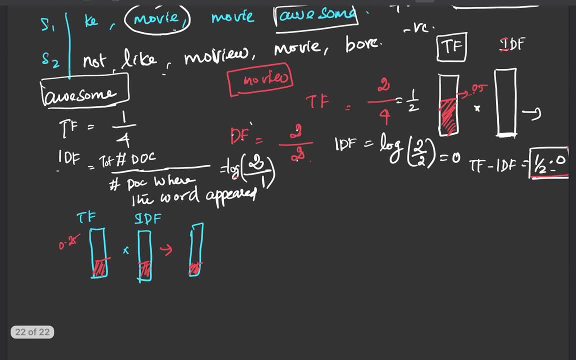 For S1 and S2, we do have the vocabulary list of vocabulary, which is which is vocabularies like movie, awesome, not bore. These are the words. And then we do have document sentence S1 and S2.. 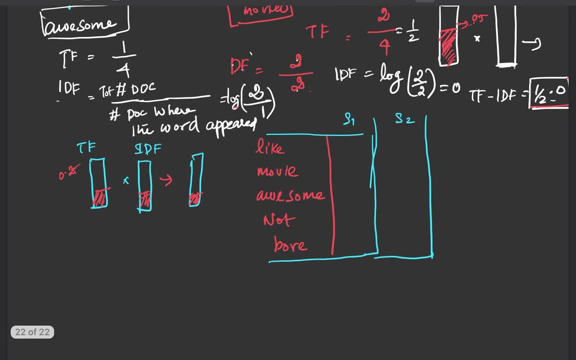 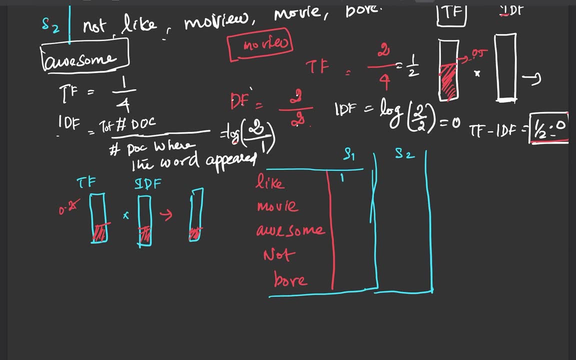 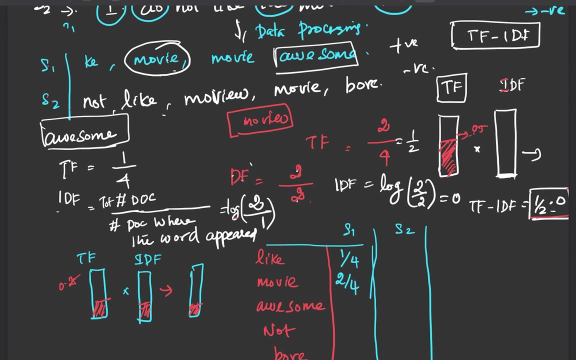 And we calculate frequency Like appeared one term. we will calculate term frequency Like appeared one out of four times Four is number of words in the sentence. This is four. And movie appeared two times Two out of four. 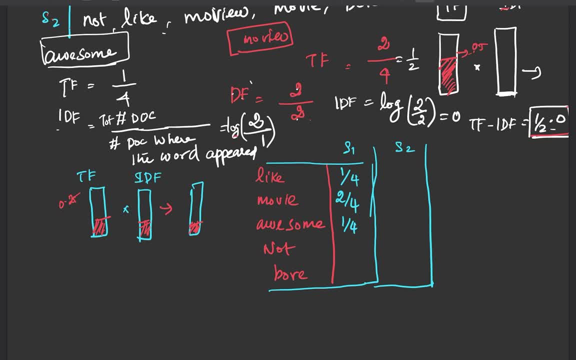 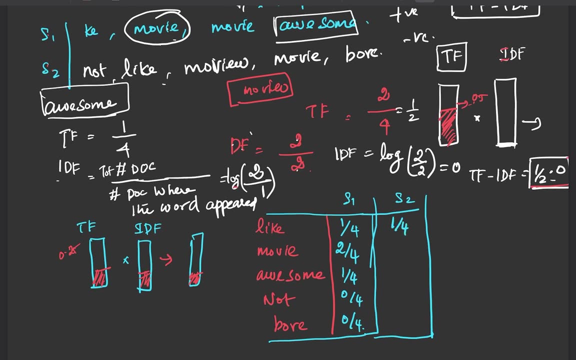 Awesome appeared one time, Not is not appeared And bore is not appeared. And then we will do the same thing for the second sentence, Like appeared one time Here. how many words Here? there are five words And we will calculate. 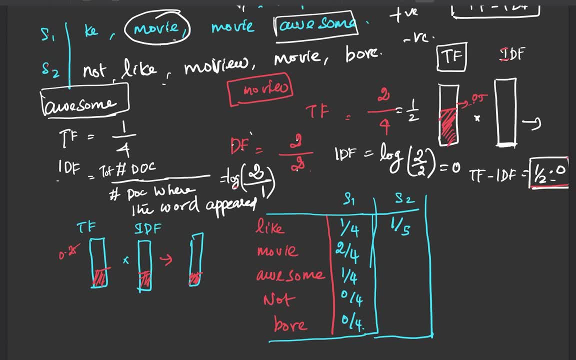 for movie two out of five. And then awesome. there is no word awesome in the second document And not one time And bore one time. So when you sum up the numerator it would add up to five. 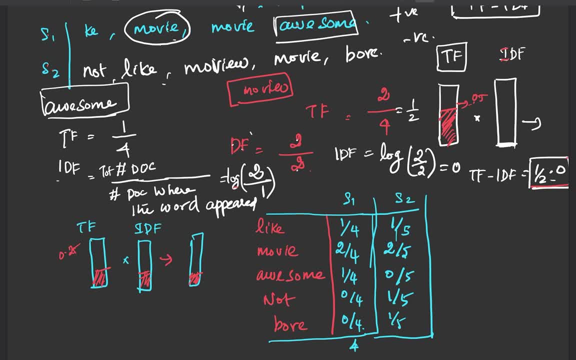 Here the total number of words here is four, here it is five. Then this is called as tf: Term frequency for document s1 and s2.. Then we will measure idf- Inverse document frequency. This is the log ratio. 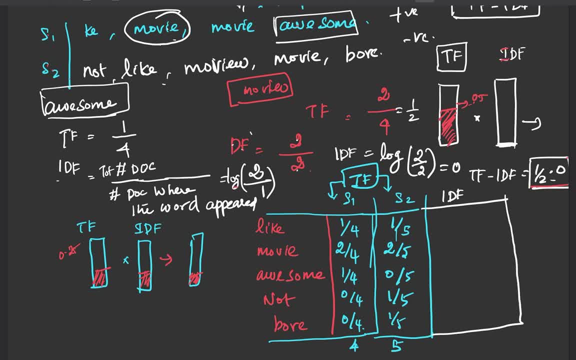 of how many times the word up Up And how many documents have that word given word. So we see like it's a log ratio. How many documents have that, like only one Which is coming in the numerator. 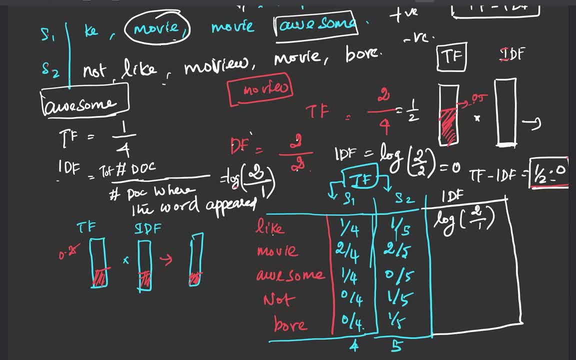 And numerator is total number of documents two by one. Same thing for movie. Movie appeared on all document, So total number of document is zero. It becomes zero. And next one is for awesome. Awesome is available on only one document. 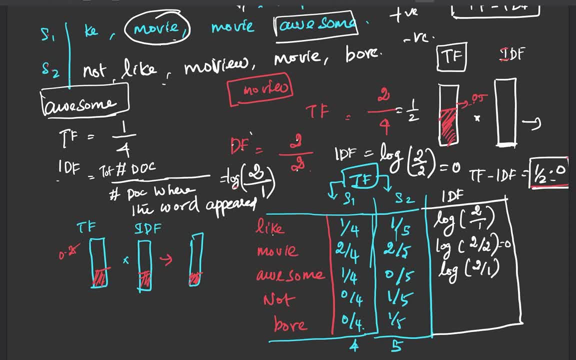 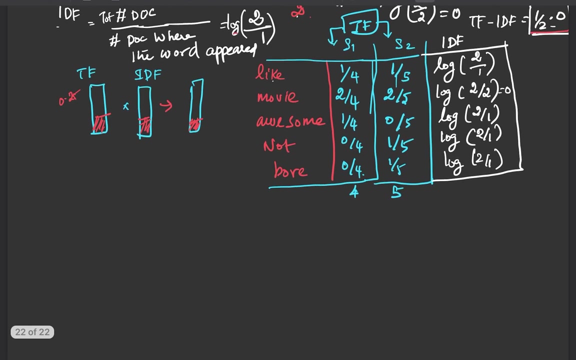 out of two, So two by one. Next one is log. This is also same And boor. Okay, Now we got these numbers- TF and IDF. Then how we extract the features, Just for S1 and S2,. 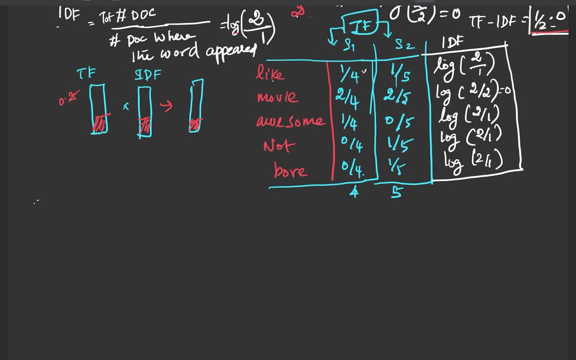 we can just multiply these two numbers. So I put like movie awesome, not boor. And for the first one, for the first observation, you just multiply one by four. log of two by one. This becomes two by four. 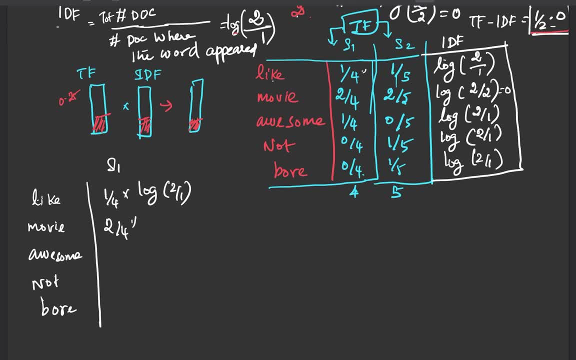 becomes this? log two by two. zero Eventually becomes zero. Awesome, One by one by four. log two, not not there. It's zero into log two, which is zero, And boor is not available in the first word. 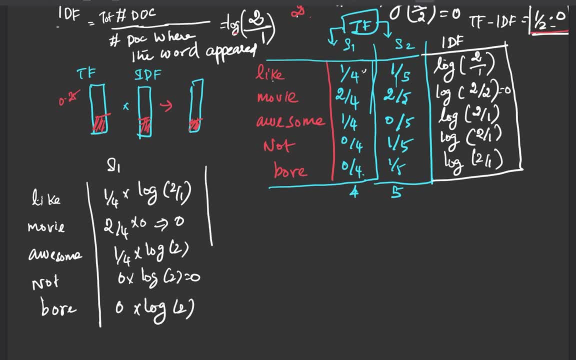 Zero, log two. Similarly, calculate the TF IDF for the document. two for every words. For like it is one by five. log of two. Here it is two by five into zero. This is zero. 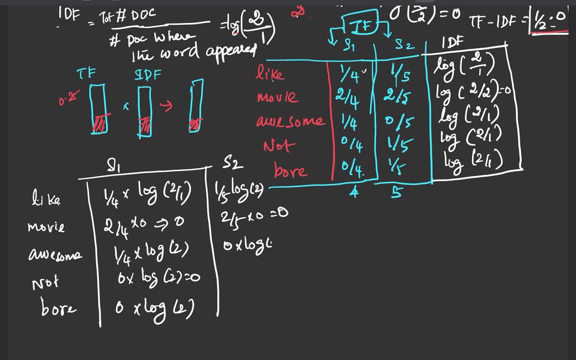 And next one is zero into log two, which is equal to zero. Next one is one by five log two: There is some number, decimal number. And next one is one by five to log two, which will have some number. 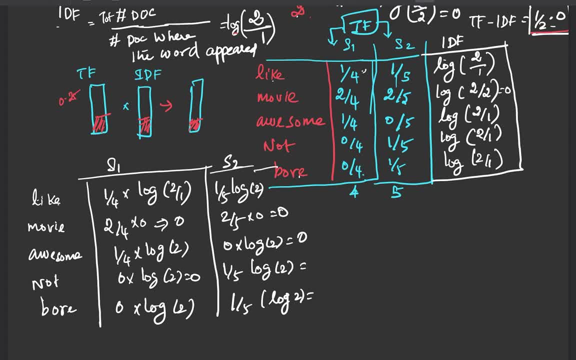 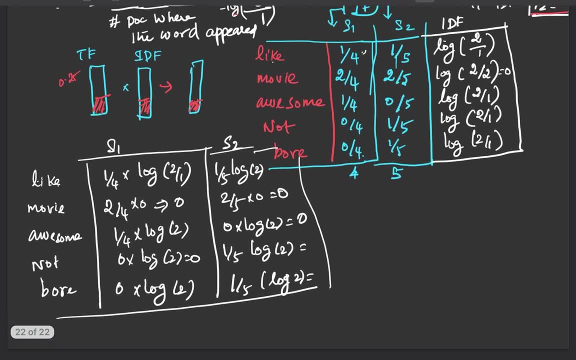 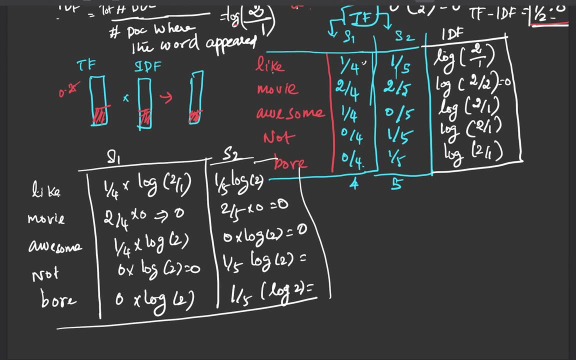 So now after calculate that, calculating these numbers, we will have features. So now how we extract the features. Features are x one x two. Here we have x one x two x three. 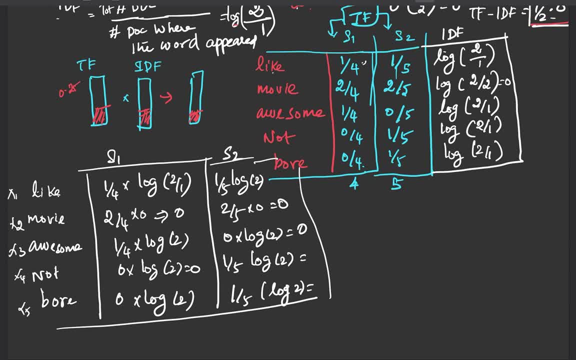 x four, x five. There are five features Now. our five features are x one, x two, x three, x four and x five, And for each sentence we have some numbers. For the first sentence, 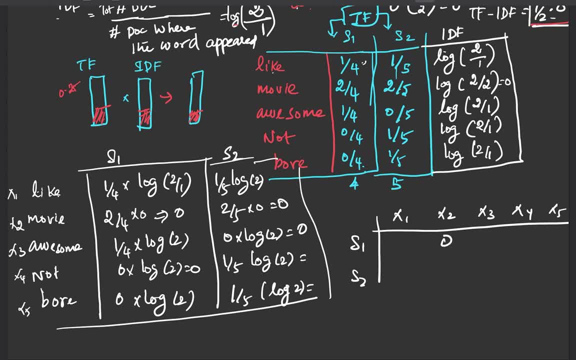 the second feature is zero And third feature is zero. Fourth one is zero. First one is one by four log two. Third one is one by four log two. Similarly for the second sentence it's: 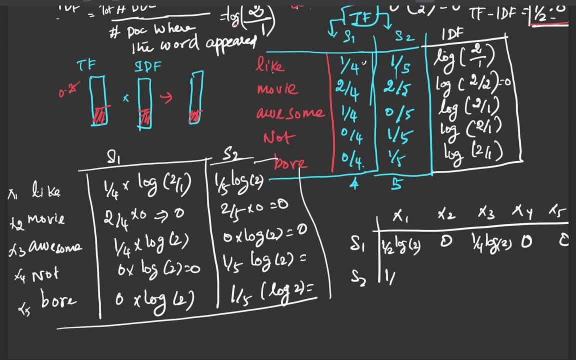 one by five, log two: Second word is zero. You know what the second word is, which is movie. Now you see, the value for movie becomes zero in both sentence And for x three. 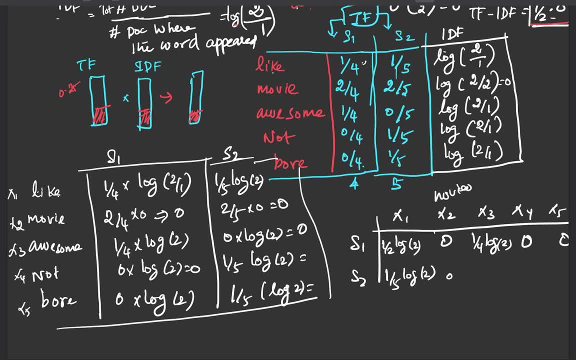 x one x two x three, which is zero. What is the word x, three, Awesome. So second sentence doesn't have awesome. And then not, which is one by five, log two. 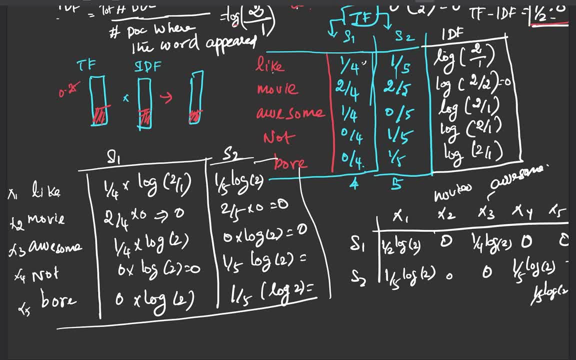 Next one is one by five, log two. Now we see how we extract the features. So this method of feature creation is in more meaningful than our previous method. bag of words. Bag of words. 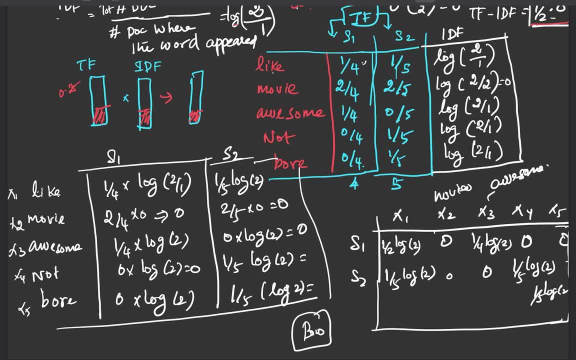 is just measuring the frequency of words within each sentence, But here not only within the particular sentence, it's also looking across all the sentence, across all the documents. So by doing so it is creating. 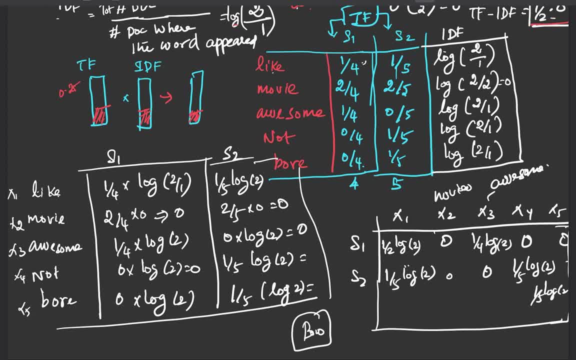 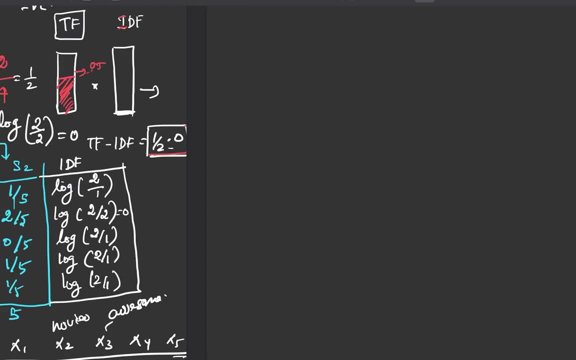 more meaningful features, which is more is that informative than the previous one. Now, do we, do we know the application of this, the famous application of TF-IDF. So one of the 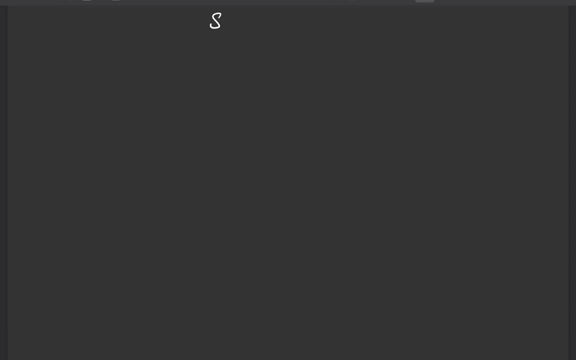 main application is search engine optimization, SEO. Actually, initially the Google search engine was using this methodology- TF-IDF, So whenever we do some search in our Google search engine, it returns. 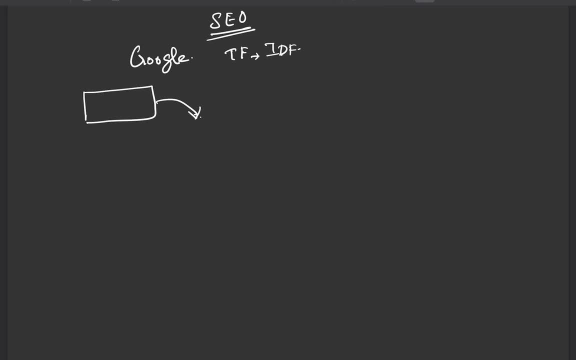 some that, some documents for us to read through. So, for an example, if I enter that, the forest honey. So how this Google search engine would works initially is 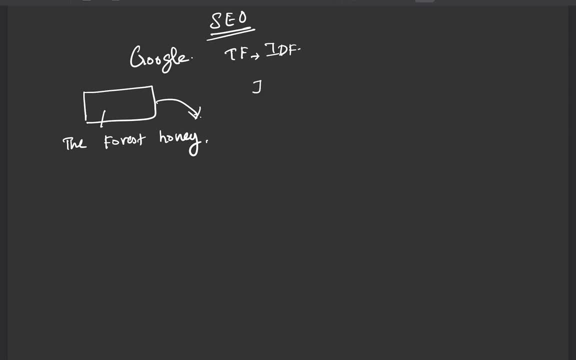 not looking for it would be searching across all the documents over the internet And look for this. keywords: the forest honey, When it was using only the this term frequency. So what do you think? 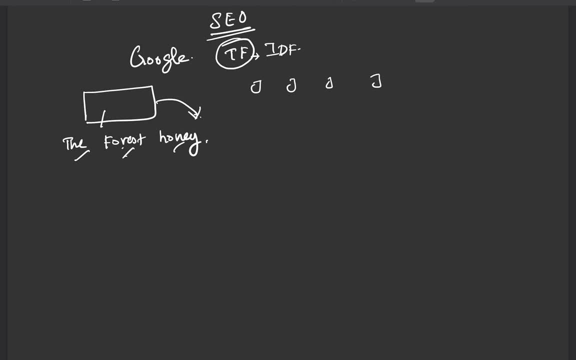 that which which kind of document would get returned When we use only the TF, when the Google uses the TF algorithm? So it would return only the irrelevant, just having this word, the, Because 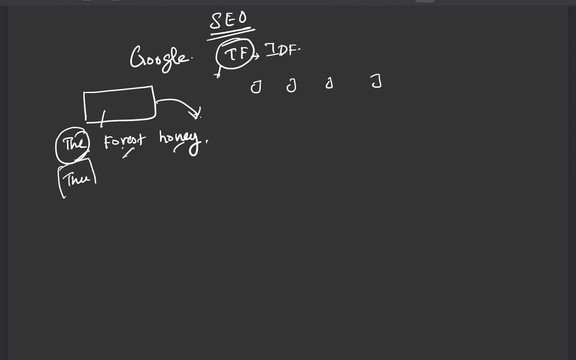 the is more common and all the documents may have more of these. this term, the rather than forest honey. So it would be returning some irrelevant document. maybe about the movie review, it may. 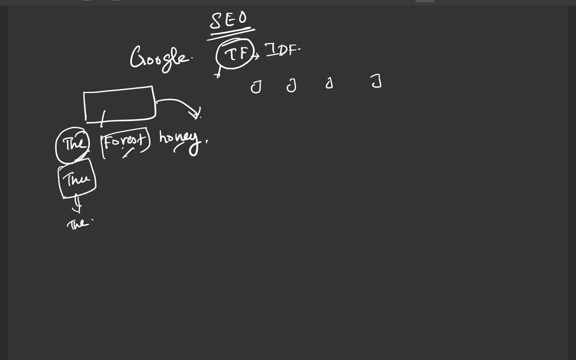 return some document about the story, maybe fairy tale story, any kind of document it can return. So when this TFS is combined with IDF, what it do is not only, it is looking for the word. 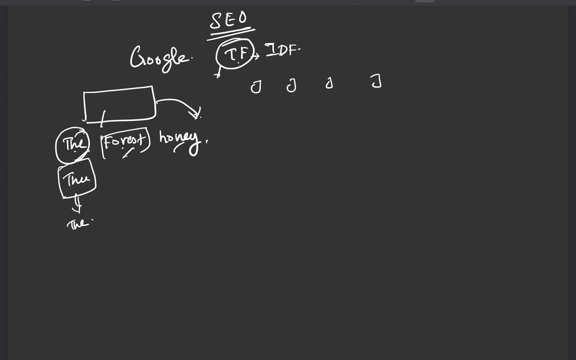 frequency of this word, the within the given document. it also see how unique the given search engine is. search words are within the document. So when, when it, when it includes this IDF, the, the remaining words. 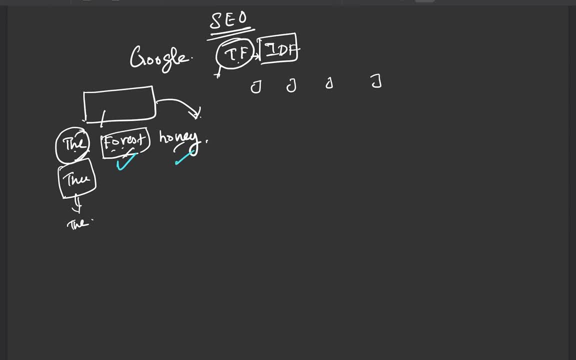 forest honey would get more importance, Because forest and honey might be more relevant to the document too. The document too may have lot of forest and honey- the word forest and honey- but not the remaining set of documents. 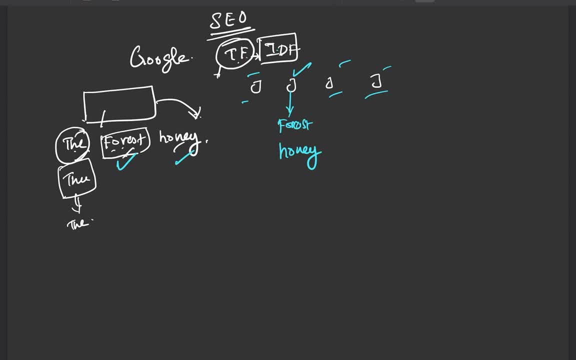 So when this TF, IDF is joined together, then it knows that this particular document too, is more important, and then search engine fetches the document forest to read through. Maybe next time when you use. 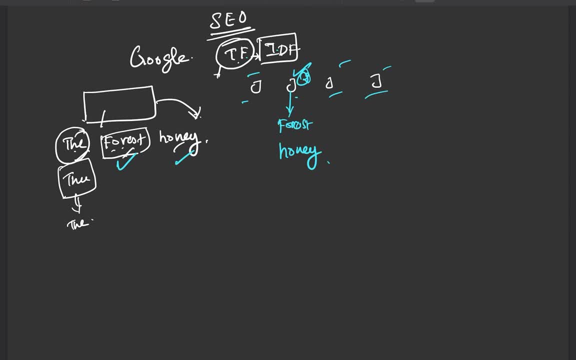 Google search engine. just interestingly, you just randomly give some keywords like this and see what type of document you get from the Google search engine. So maybe the combination of two words like forest. 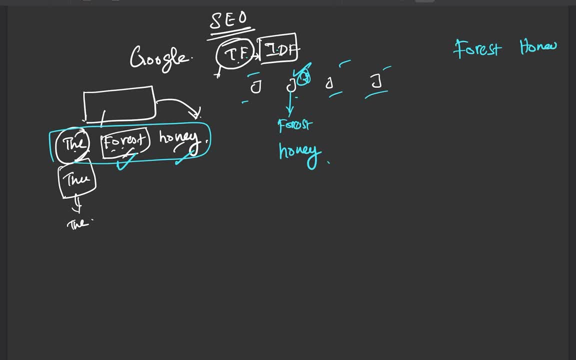 honey, honey, and then use some words forest honey, and then use some words forest monkey, and then maybe monkey food, and see what type of document you get. Another one is food taste. 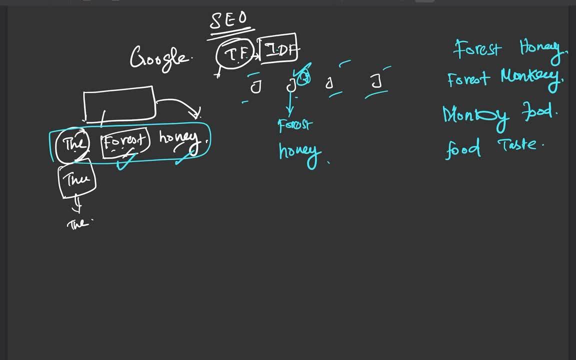 So we can. we can combine different words of words together and then see what type of document Google returns. So this is the older way. Now the Google search engine has been updated a lot, It seems like.